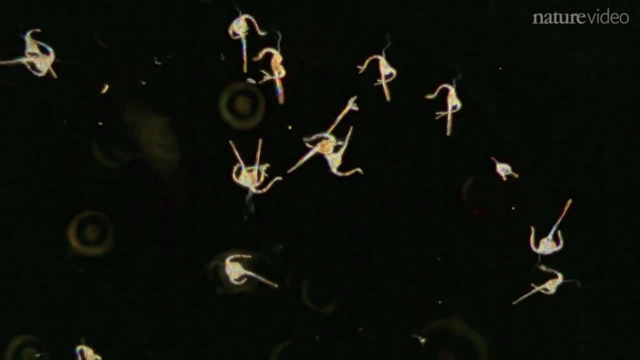 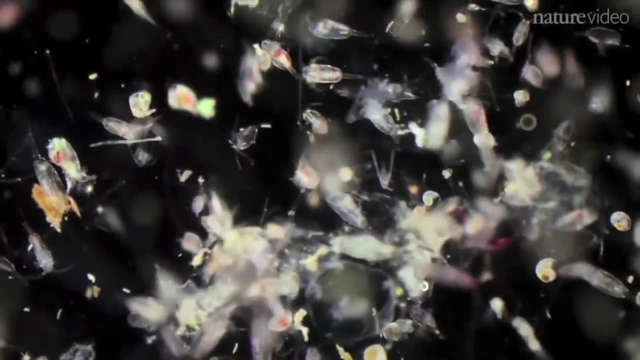 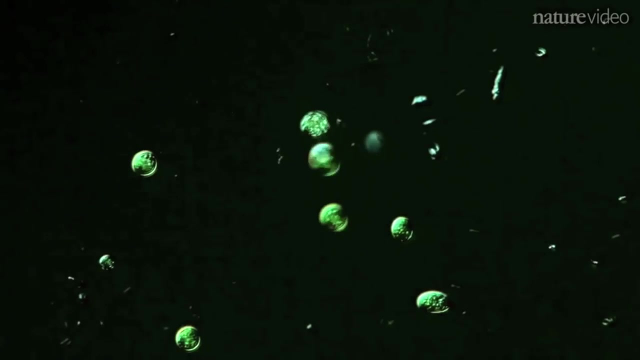 10 meters of the oceans. They live as single cells or grouped together in chains, and they can photosynthesize just like plants on the land. It has been well observed that phytoplankton can control their movements in the water and move towards light and nutrients. The phytoplankton 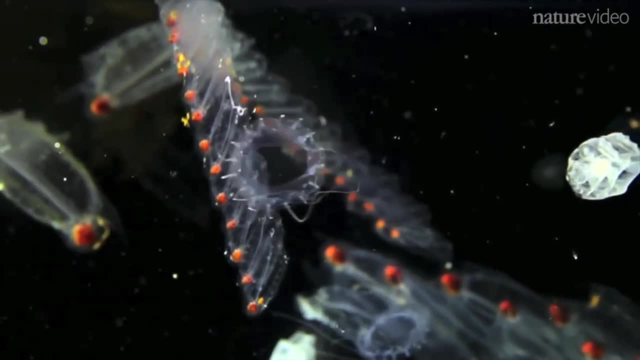 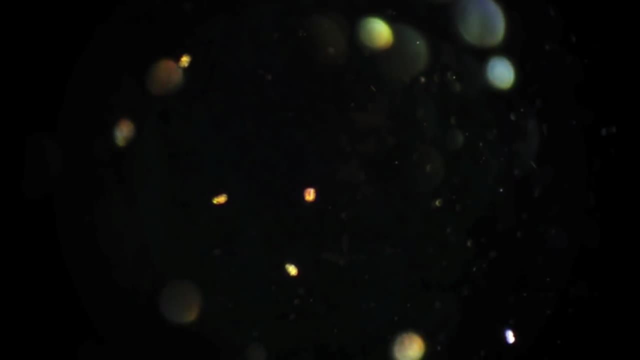 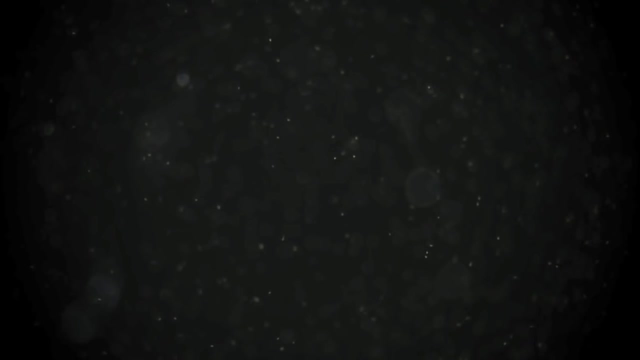 can clearly sense the predator is there. They flee even from the chemical scent of the predator, but are most agitated when sensing a feeding predator. So plankton feed on phytoplankton and are then eaten by larger zooplankton fish, larger fish and so on. Plankton are at the base of a complex 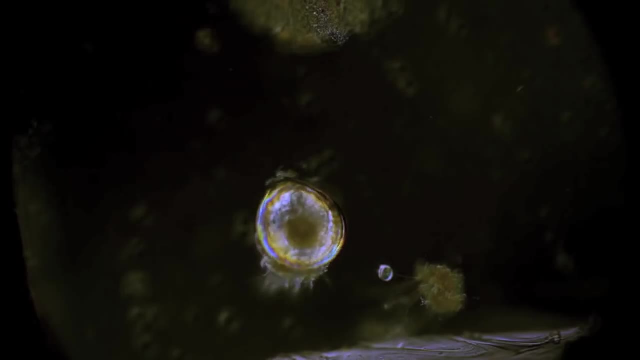 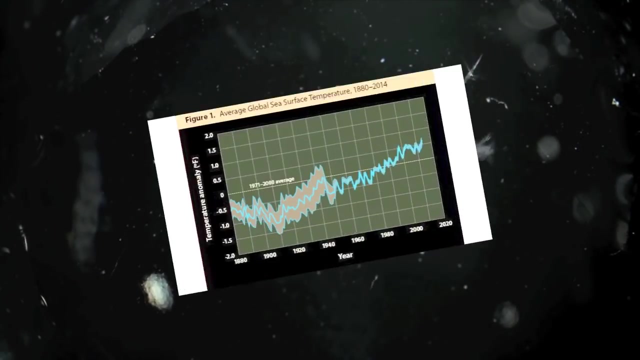 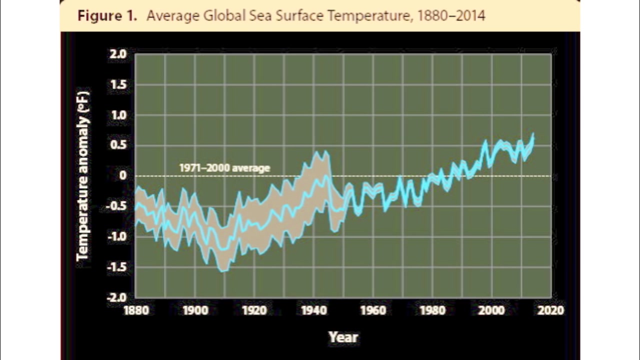 aquatic food web. Sea surface temperature is expected to increase 2 degrees Celsius on average globally in the next 20 years. Some of the consequences of this increase include changes in ocean circulation and higher water column stratification, thus affecting the nutrient availability for the growth of marine vital plankton. 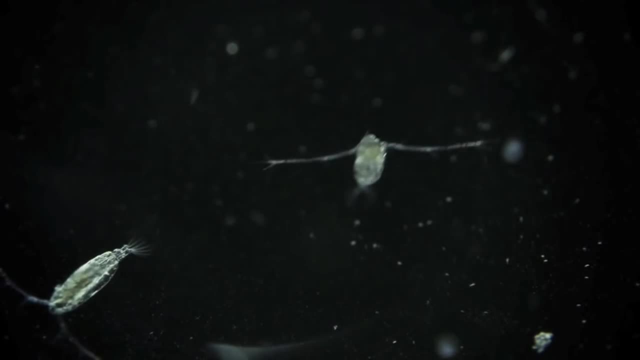 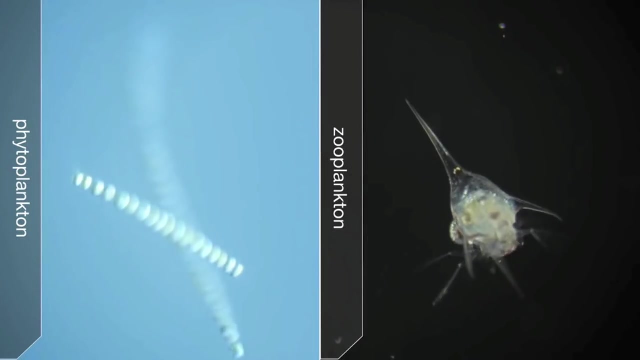 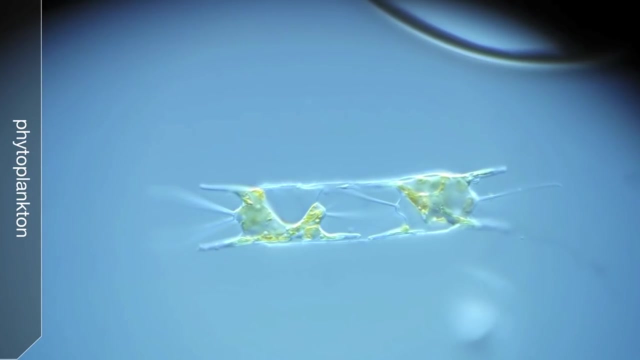 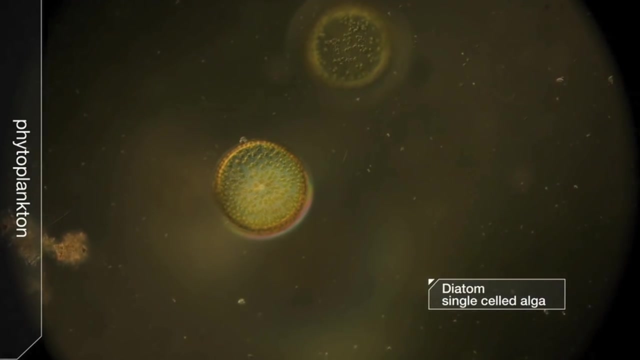 Globally, it is estimated that the sea temperature rise will cause phytoplankton and zooplankton biomass to decrease by 6% and 11%. Conservation efforts to save phytoplankton. Eat eco-friendly fish. Limit your use of plastics. disposables and single use projects. 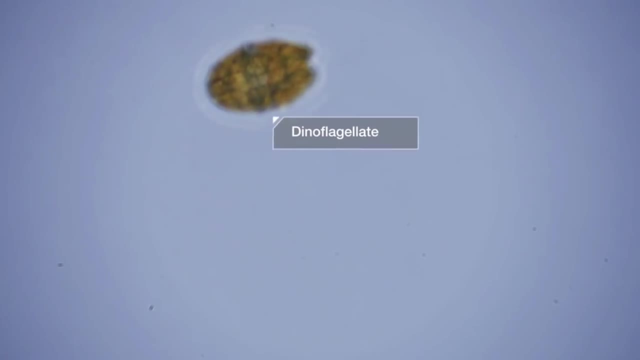 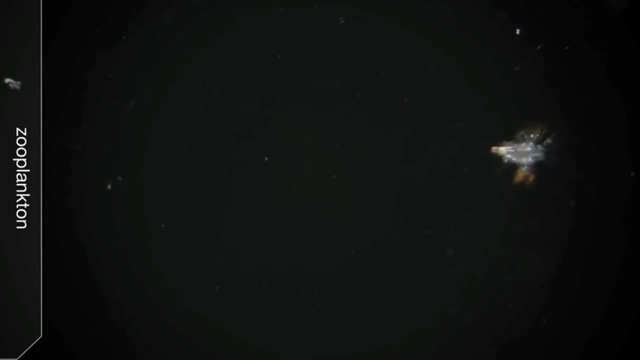 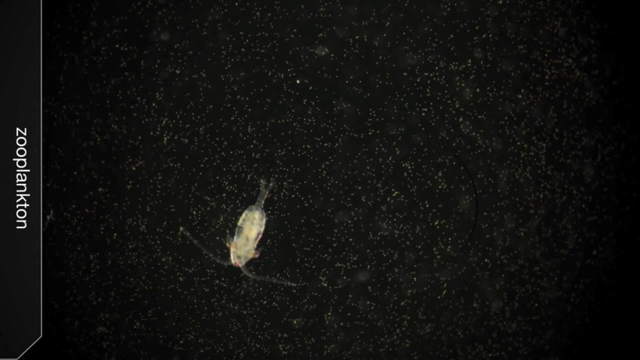 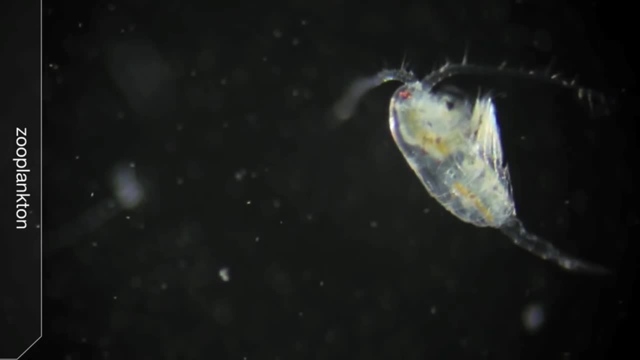 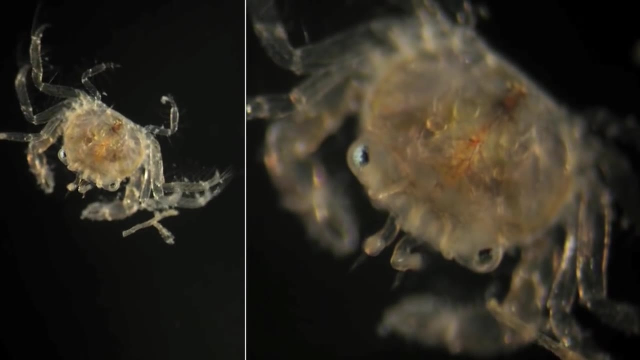 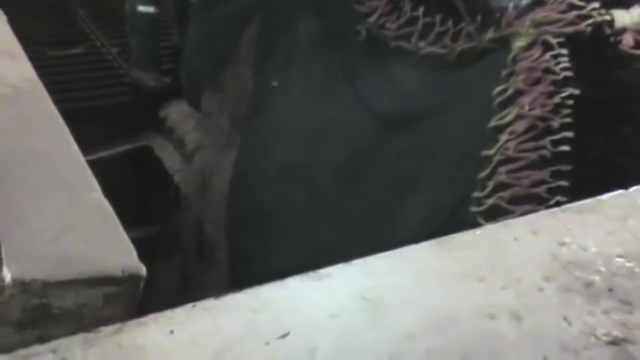